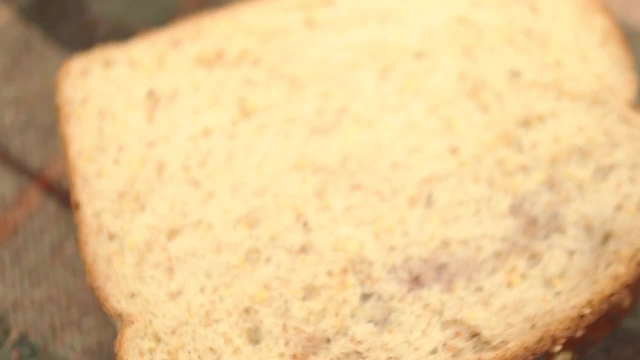 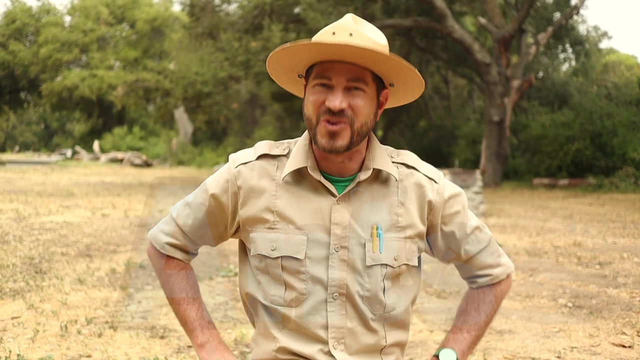 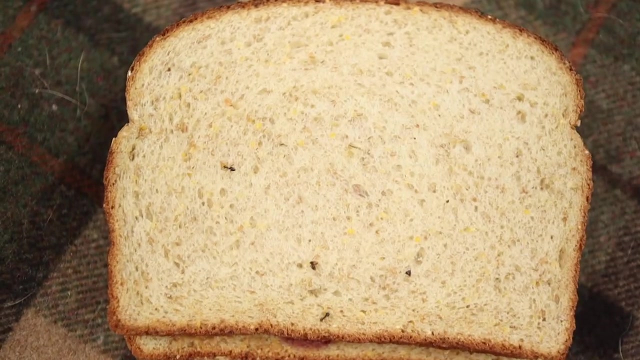 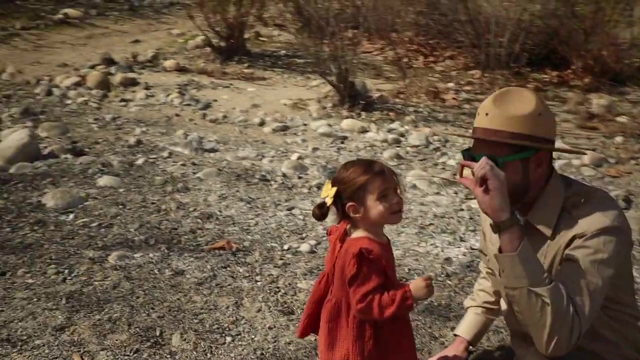 crawling all over our food. they're actually a very helpful part of nature. So today let's talk about the social, hard-working, super strong world of ants. If you ever want to know what makes a tree grow tall, a white turtle wears a shell on its back. 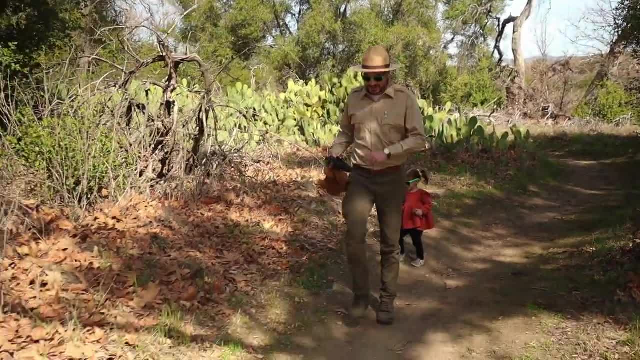 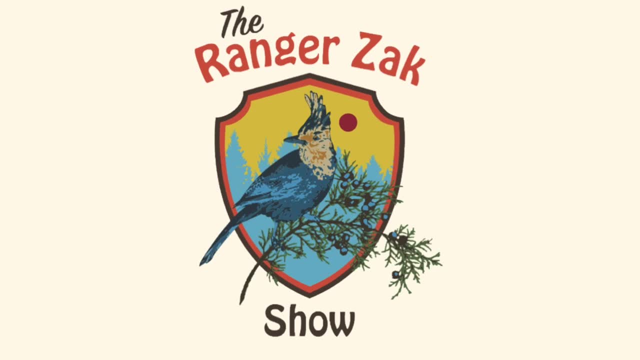 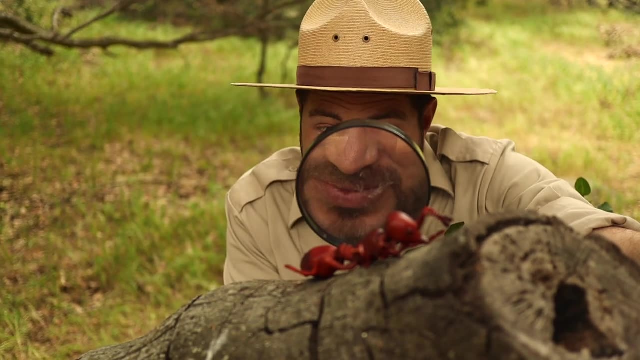 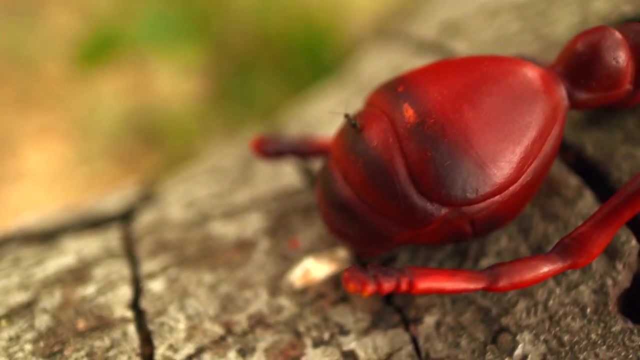 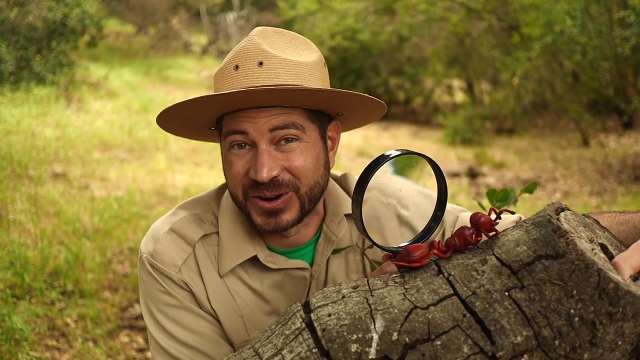 To get your hiking boots and a walking stick. come along with Ranger Zach. Come along with Ranger Zach. It's the Ranger Zach Show. Oh, cool Now. just about everybody is familiar with the common house ant, but did you know that there are over 12,000 species of ants found throughout the world? While some of these ants can bite or 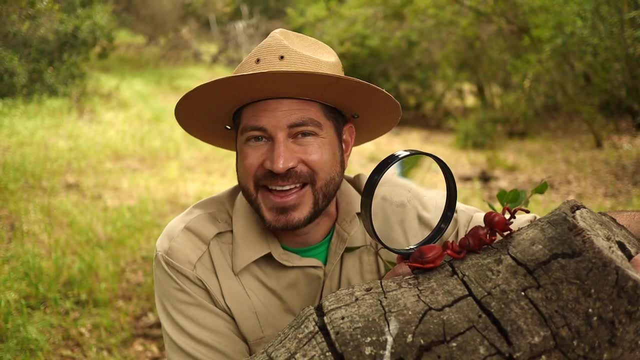 sting. most are pretty harmless when it comes to people, And ants can come in many different colors, shapes and colors. Some of them can be red, some of them can be yellow and some of them can be blue. Some of them can be red, some of them can be yellow and some of them can be blue. 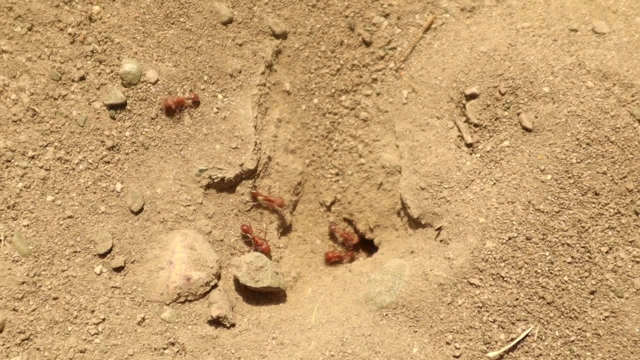 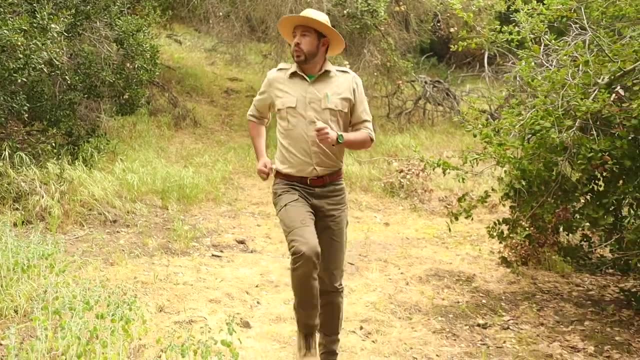 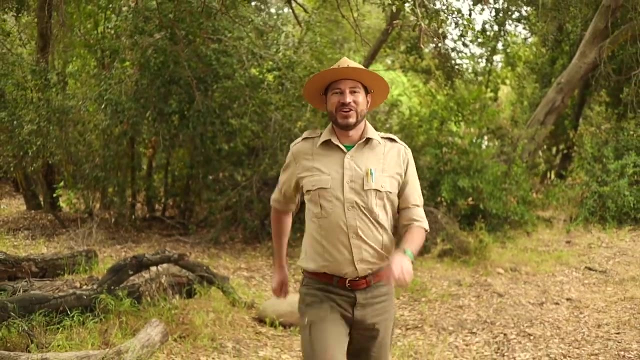 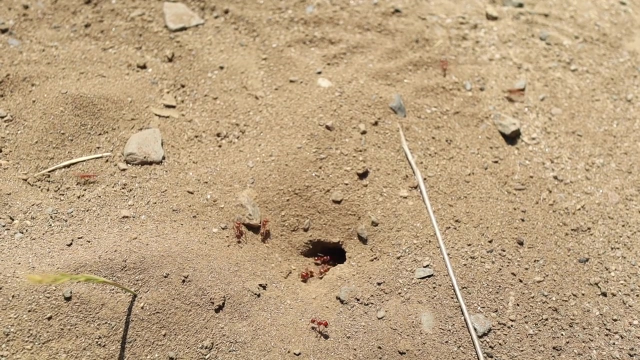 But they all live in large communities called colonies, And everything they do is for the good of one another and the sake of the colony. Ready Halt, A single ant community, may be home to 10,000 ants, and sometimes colonies combine to work together. 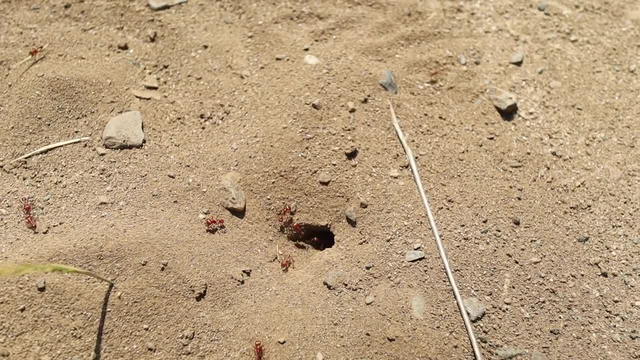 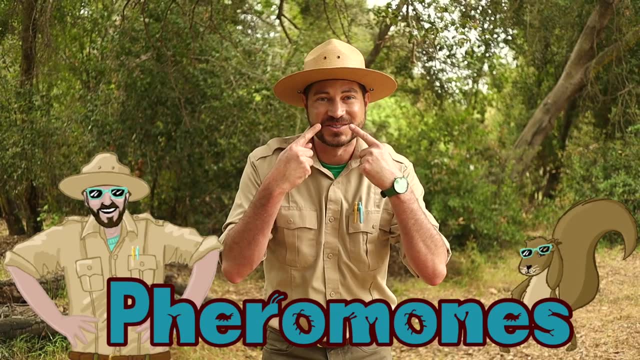 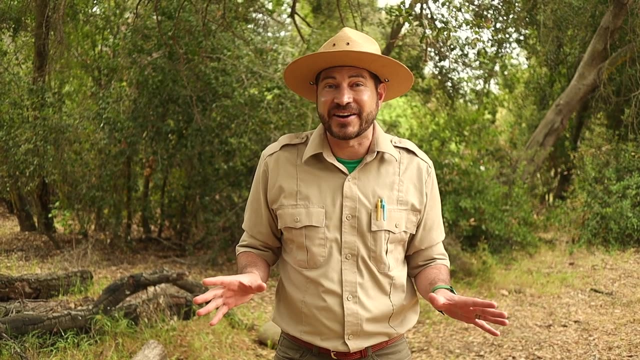 Creating super colonies of millions of ants. Now that takes a lot of teamwork, And to help them communicate, ants use special smells called pheromones. Each smell has a specific message. Like when foraging for foods, ants leave a trail of pheromones pointing them in. 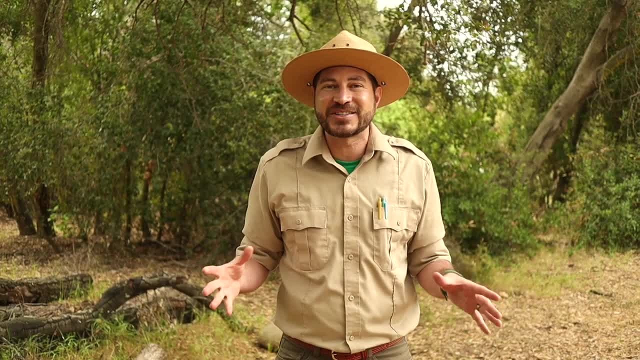 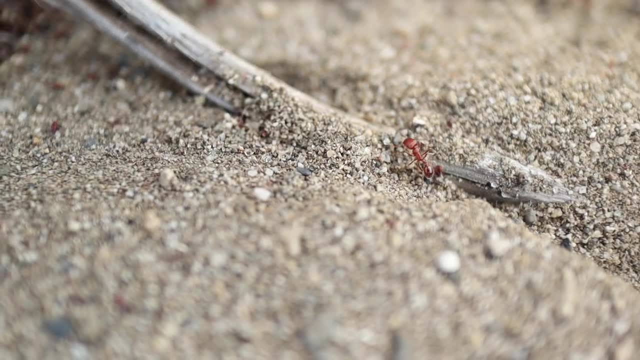 the direction of the goods, But different pheromones can be left for all kinds of different messages, Like when there's danger nearby, when it's time to move the colony, or time to move the food, Or when it's time to raise new queens. 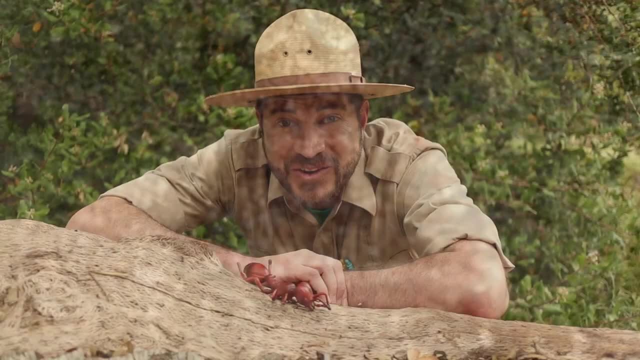 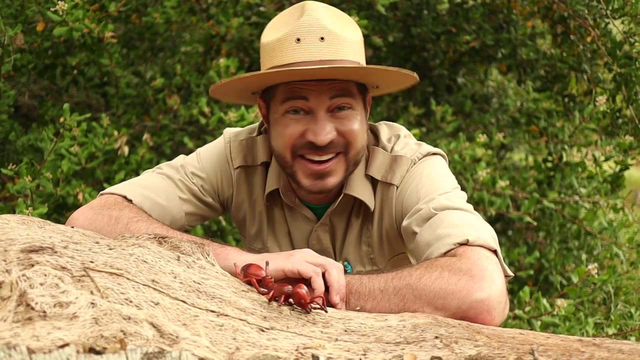 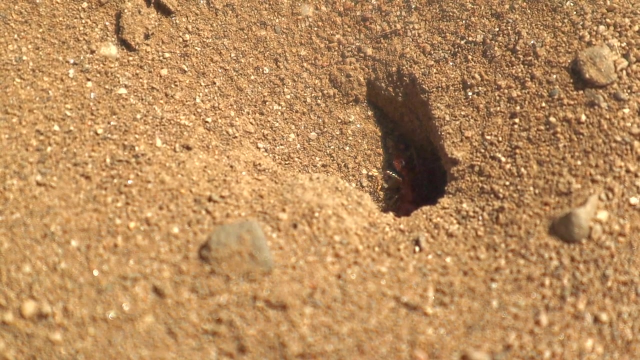 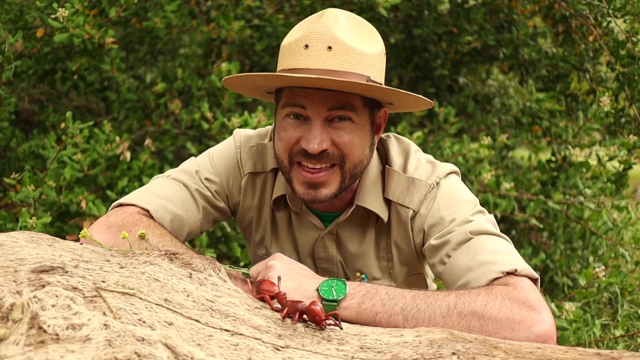 Once a message is sent, ants pick it up, not using a nose, but with their antenna. Oh boy, what's that smell? And even though ants don't have a nose, they have a very strong sense of smell, Four to five times stronger than most other insects. Oh, you're poochy. 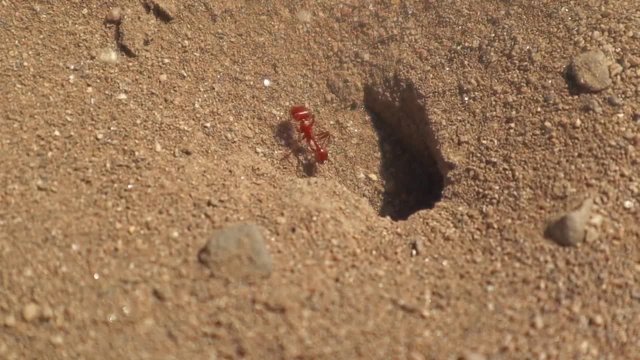 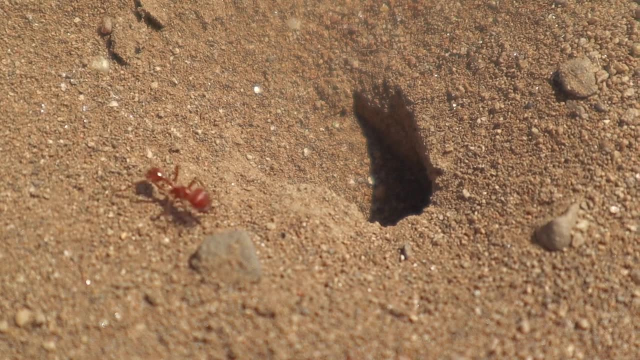 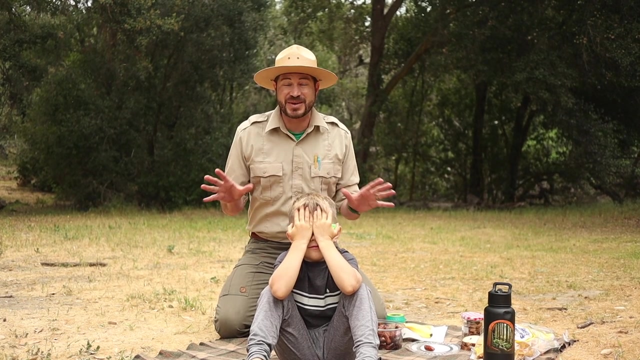 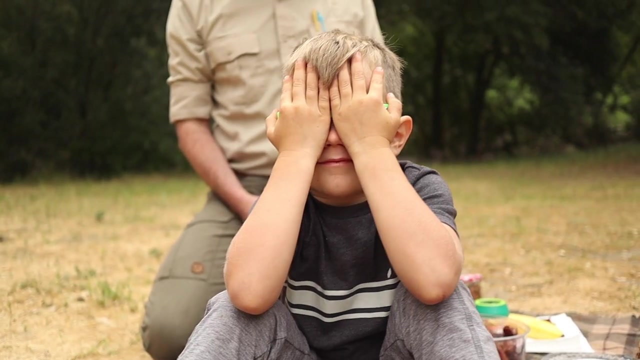 Okay, Junior Rangers, to give you an idea of what it's like to see the world using smells, we're going to play a game with Junior Ranger Tommy. With his eyes closed, he's going to play Guess the Smell. Okay, Junior Ranger Tommy, are you ready to play Guess the Smell? 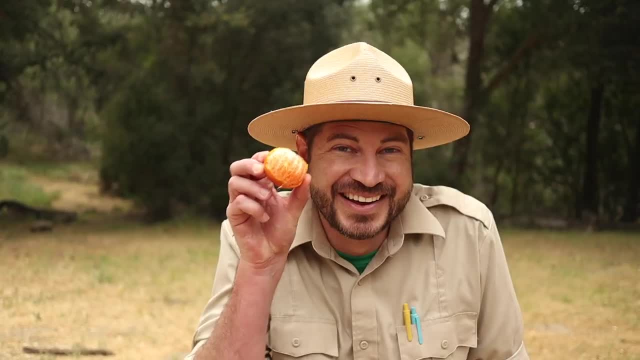 Yeah, Here we go. Guess the smell. Um, pumpkin A pumpkin. No, Guess again, Orange An orange. He got it right, Good job, Okay, Junior Ranger. Tommy, are you ready for another one? Yeah, Okay, here we go. Guess the smell. 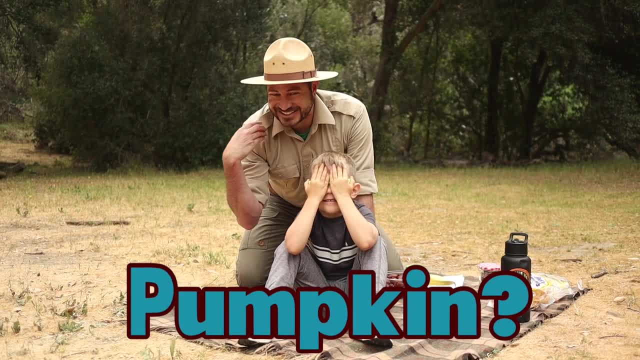 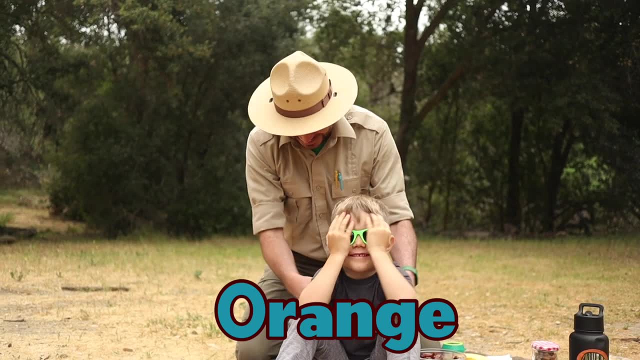 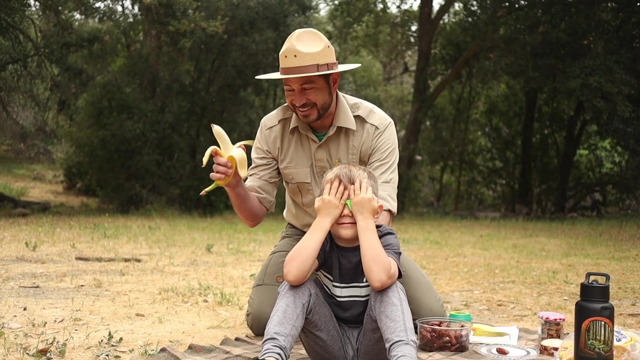 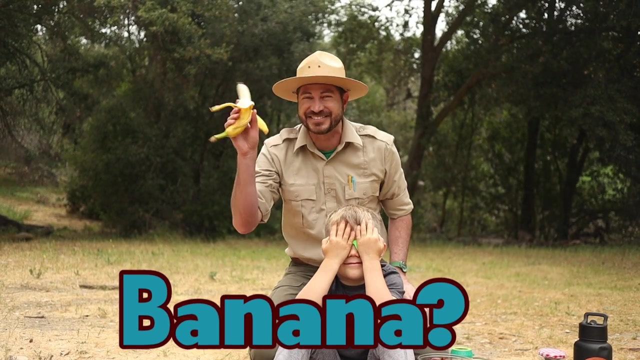 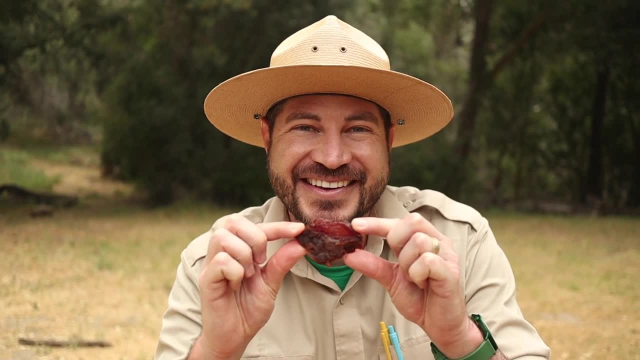 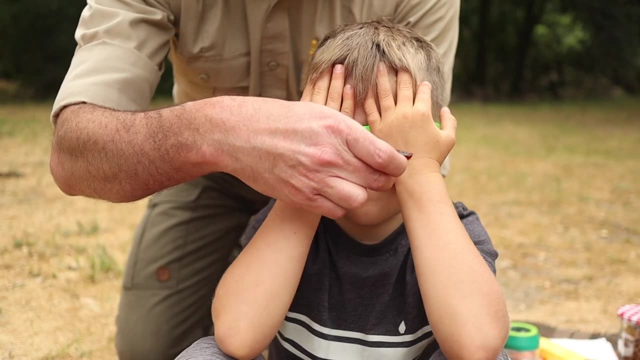 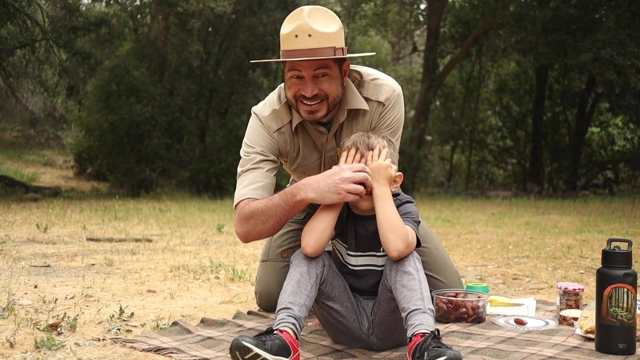 Ah, Ah, Ah, Good job, He guessed it right: A banana. Okay, this one's going to be a little tricky, Are you ready? Mm-hmm, Antelope, Not antelopes. It smells like a meat, like a kind of type of meat. 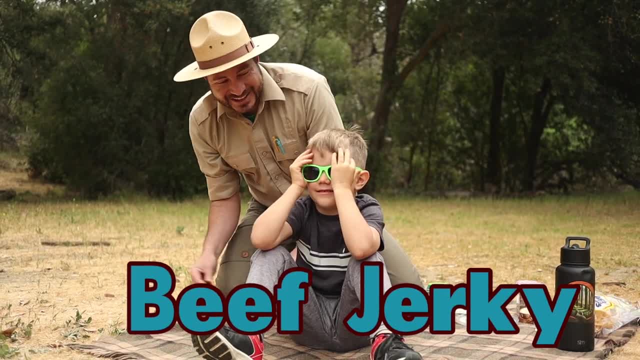 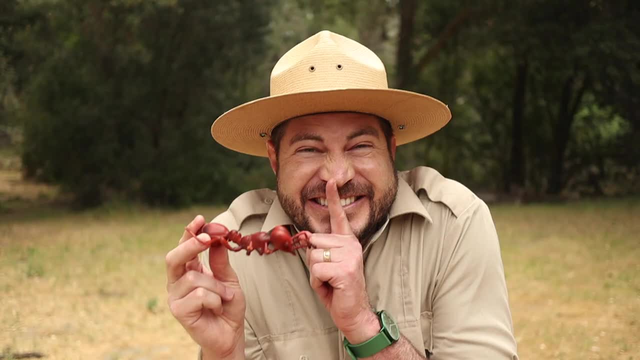 It is a type of meat, It's beef jerky Here. you want a piece? I want a piece. Oh Oh, Oh, That's a good one. Good job. Oh, Oh, Oh, Good job, Good job. 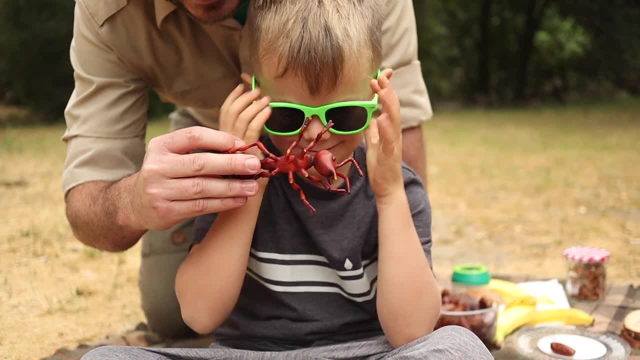 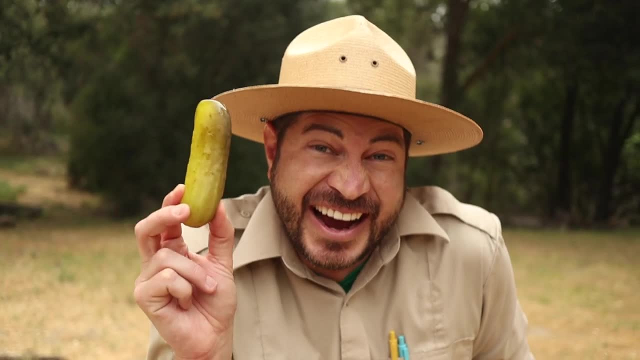 How about this one? Okay, Junior Ranger, Tommy, are you ready? Yes, Smell this one. It smells like a meat, like a kind of type of meat. Ah, Aah, Aah, Aah, Aah. 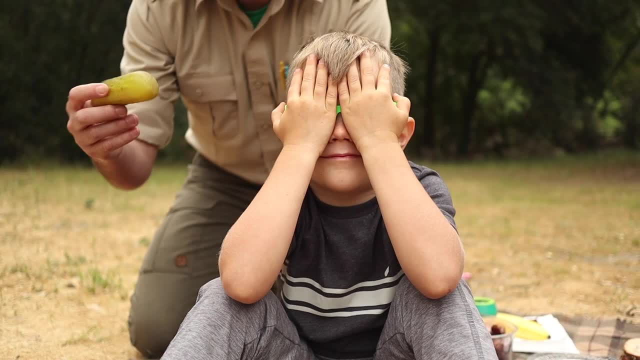 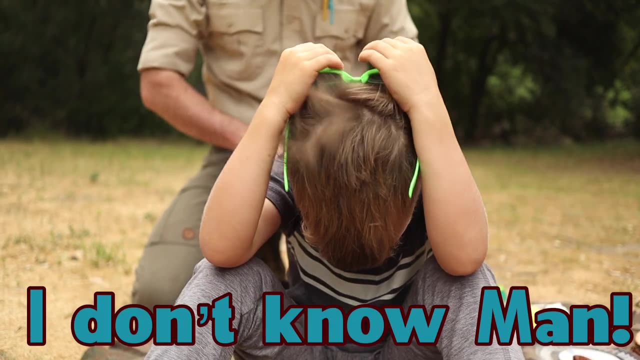 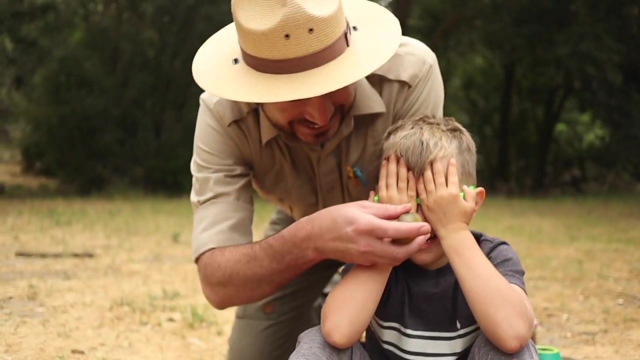 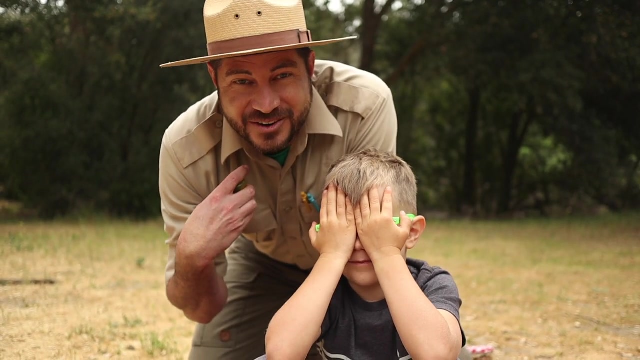 Okay, Junior Ranger, Tommy, last one, You ready? Mm-hmm, Here we go. the smell i'll talk. nope, i don't know, man, i'll help you out. here we go. keep them nice and close. it smells like something i ate before, but i don't know what it is. take one more big whiff. 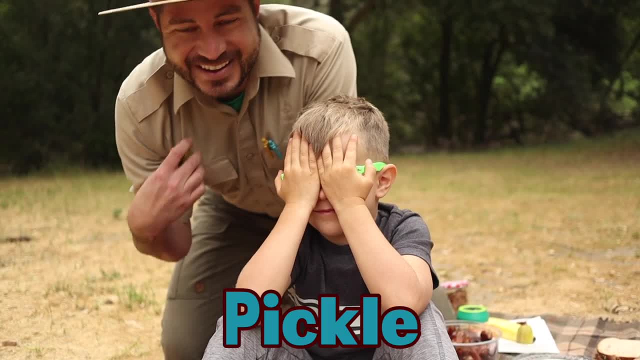 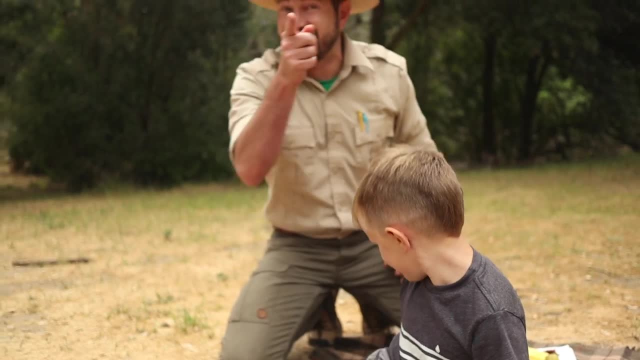 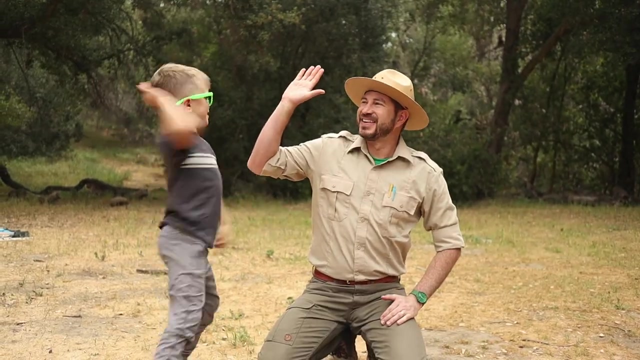 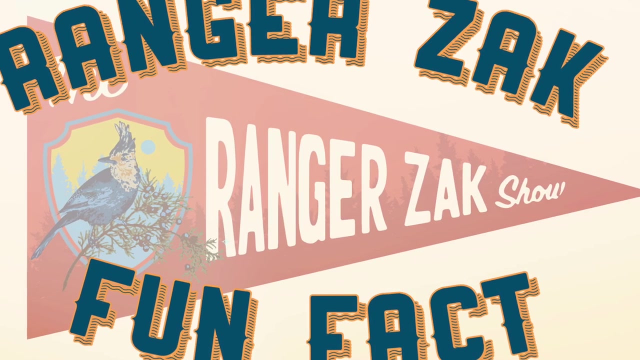 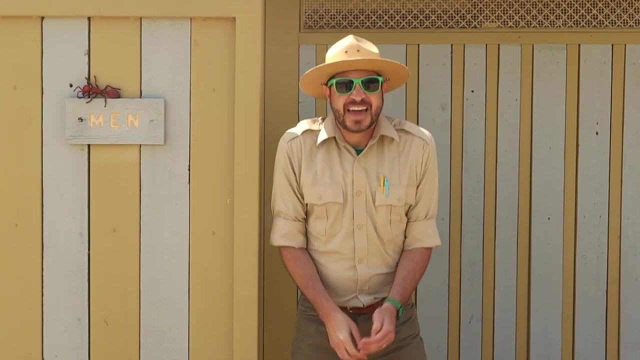 i don't know, it's a pickle. good job, junior ranger tommy. thanks for playing. guess the smell. do you want to have any of it? are you ready for your rangers act? fun fact: well, here it is. ants are pretty particular poopers and they have bathrooms in their underground nests when an ant needs to poop. 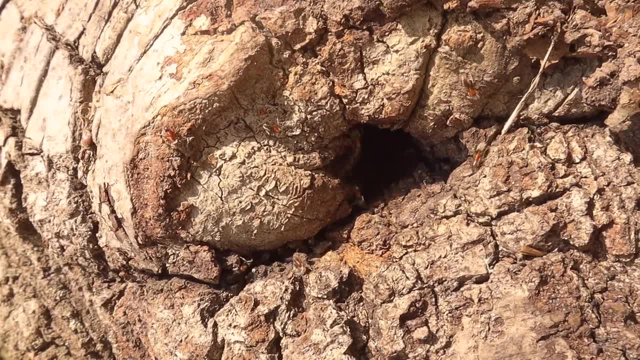 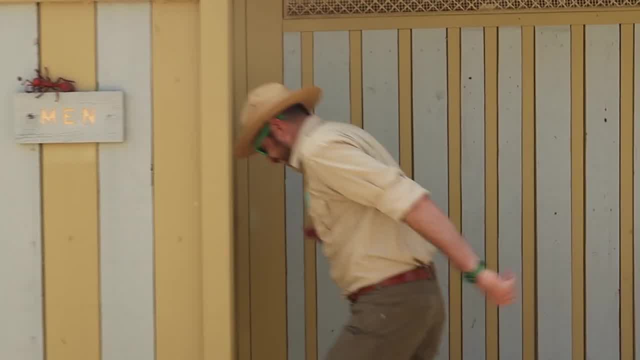 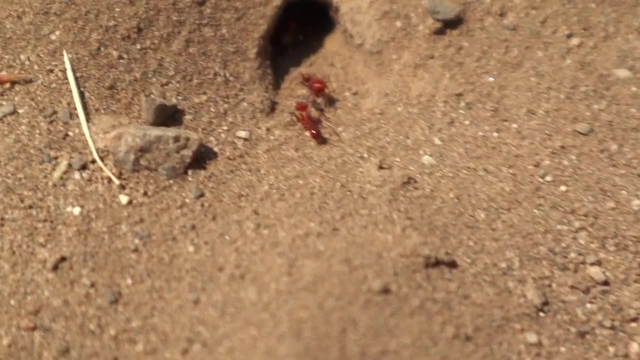 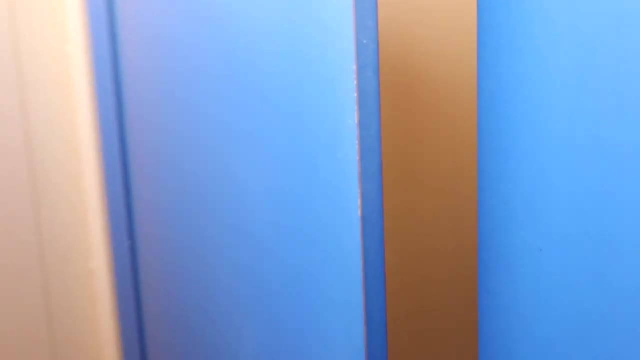 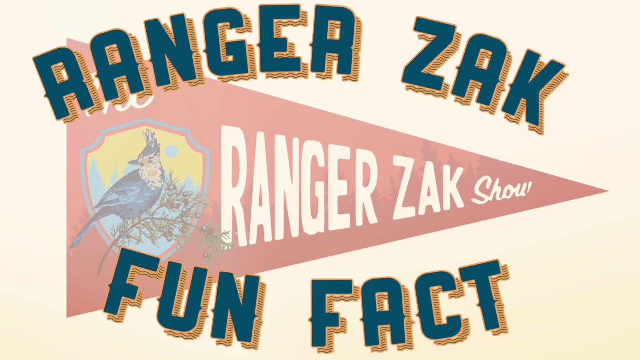 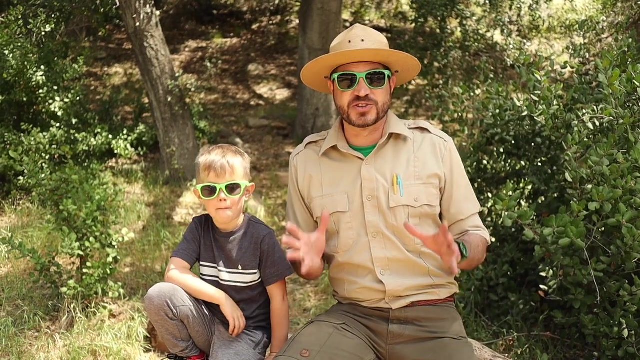 underground. they all go in the exact same spot, and it's usually against the wall or in a corner. researchers are still trying to figure out the reason for this, but all i know is i really gotta go get out of here. ants are super strong too. we're talking like super ant strong. in fact, they can lift 20 times their own. 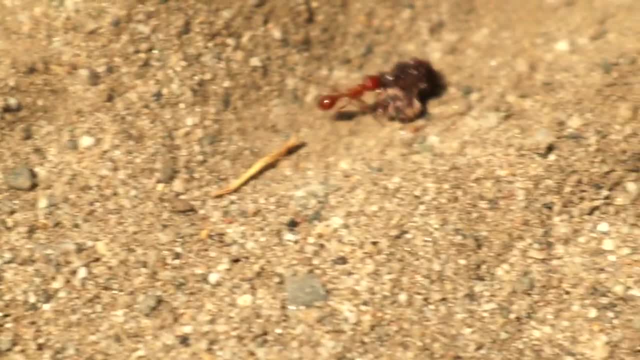 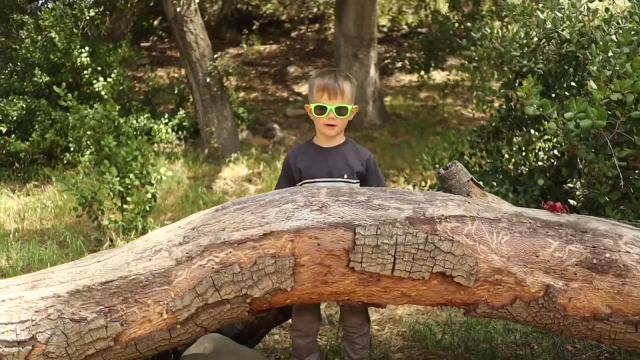 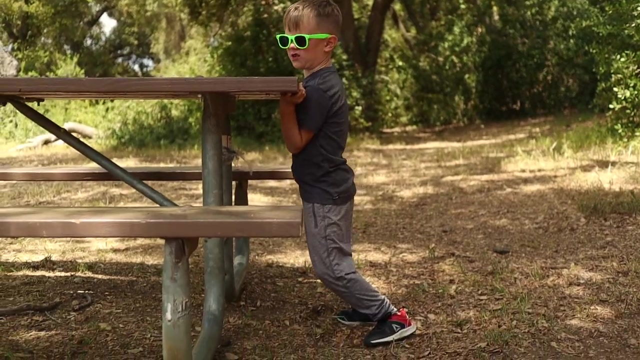 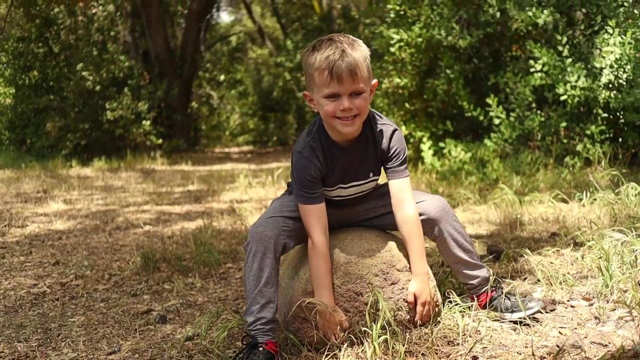 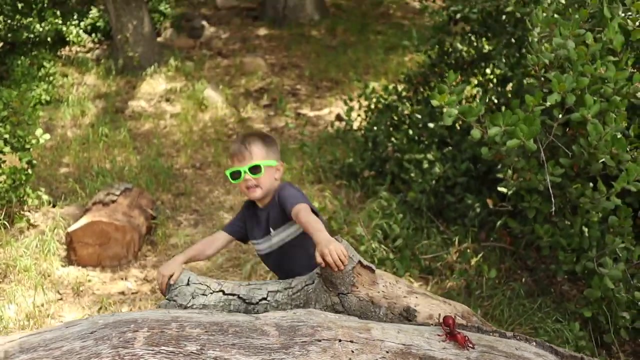 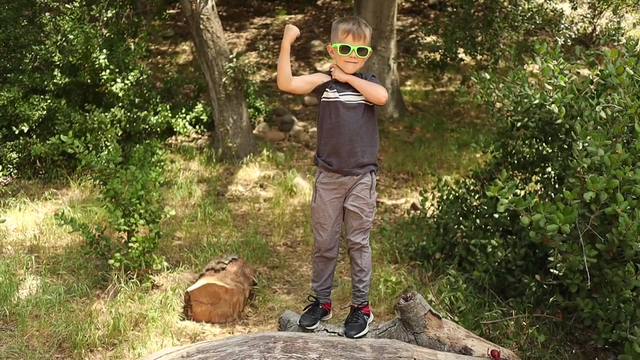 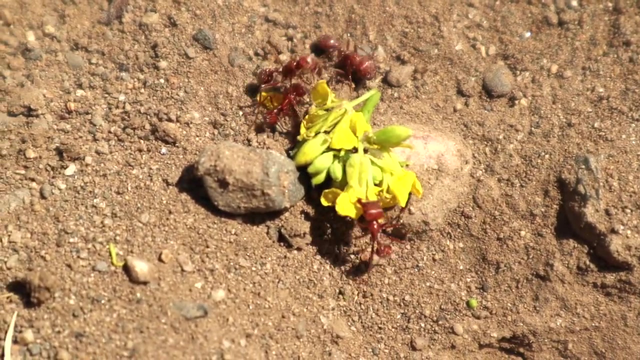 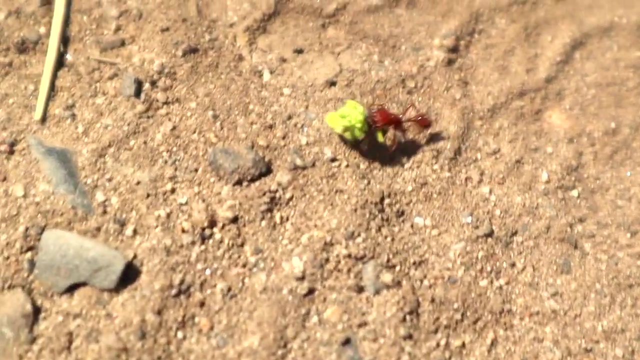 body weight. that would be like junior ranger tommy trying to lift a truck. let's see how he does and if he would ever cut it as an ant, go ahead. i almost got him. i can. i moved it cute. That's not the only strange feature on an ant's body. 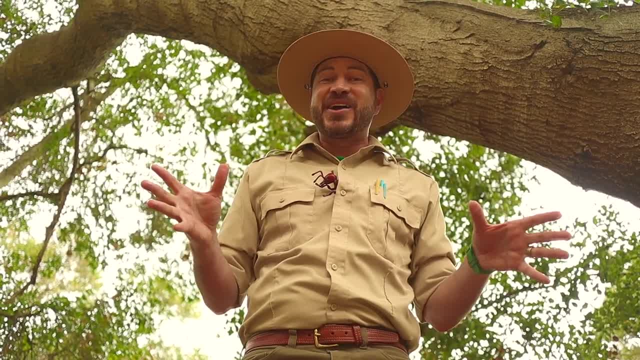 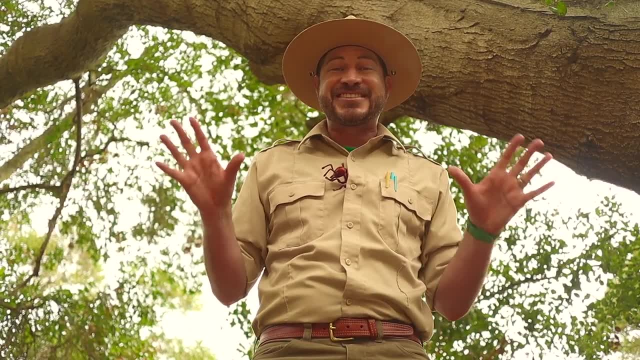 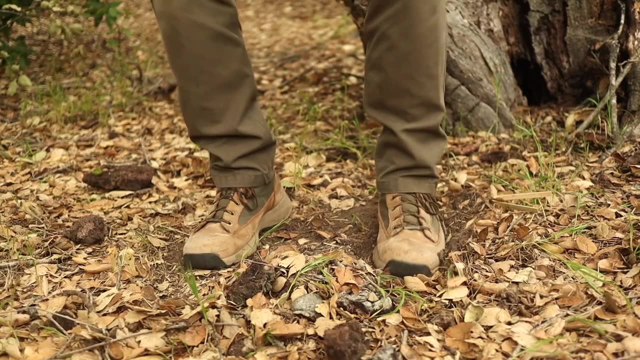 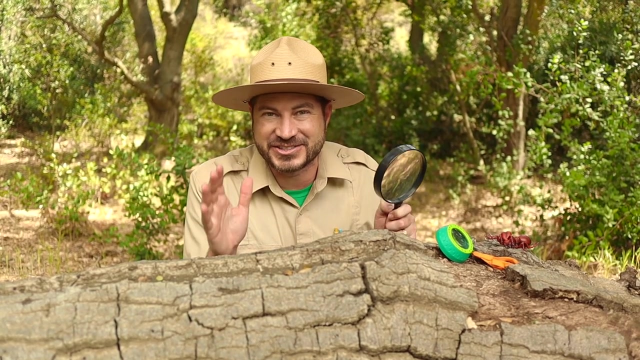 Ants don't have ears either, but they can sense vibrations in the ground using their feet and using tiny hair-like structures called sensillum. Let's send a message to all the ants nearby: Look out below. All of these special adaptations help the ant colony to survive. 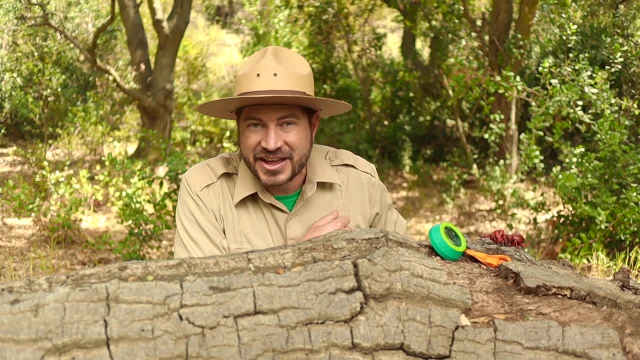 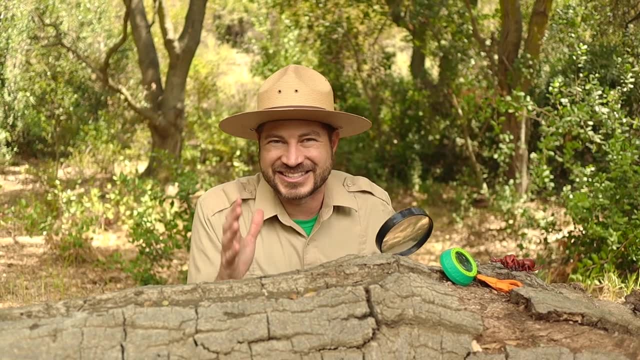 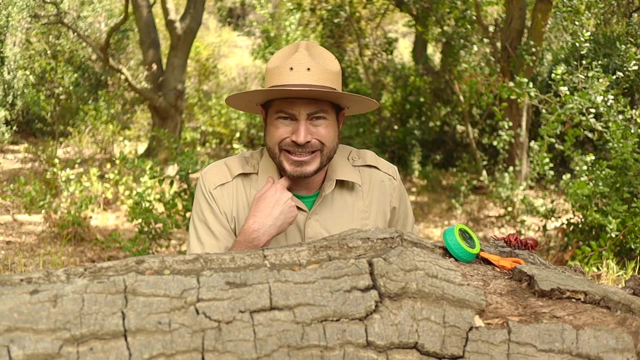 And in each colony there are three different types of ants. The queen ant- ooh, this tea is delectable. Her only job is to lay millions of eggs. All the male ants live underground with her And theykeep her company. All the other ants in the colony are females. In fact they're sisters And they're the worker ants. Their job is to take care of all the chores inside the colony, like foraging for food, building tunnels, taking care of baby ants and defending the colony from enemies. 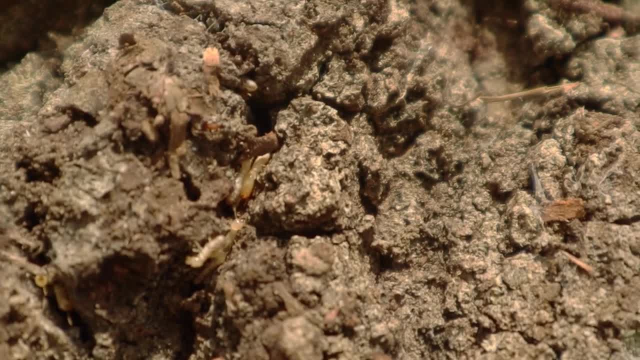 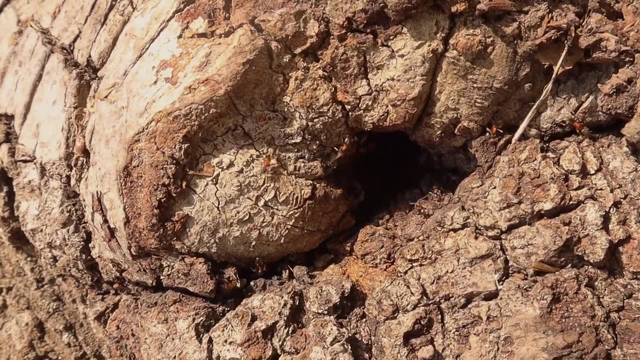 And speaking of defending their colony, These are the ant colony, These are termites, And they moved in just a little too close to these carpenter ants, And although carpenter ants are not dangerous to people, they don't exactly play nice with. 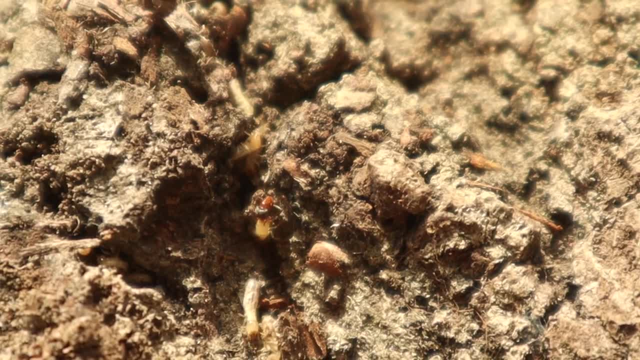 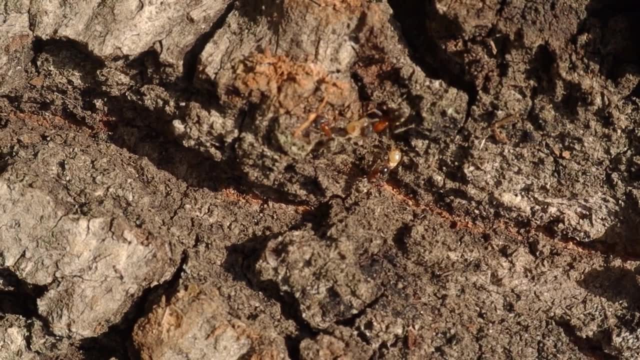 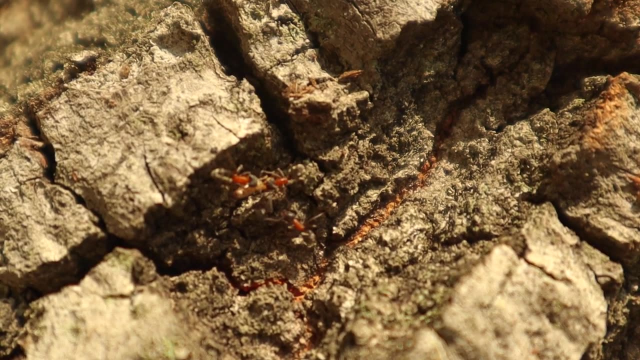 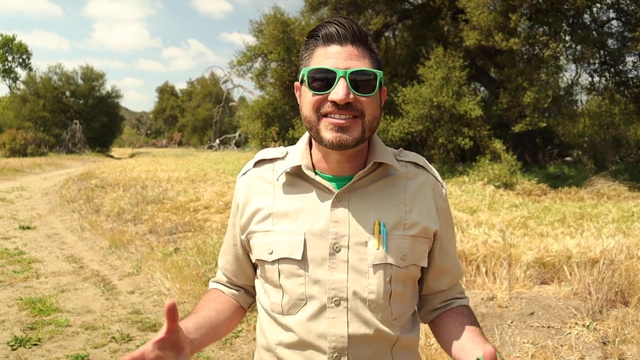 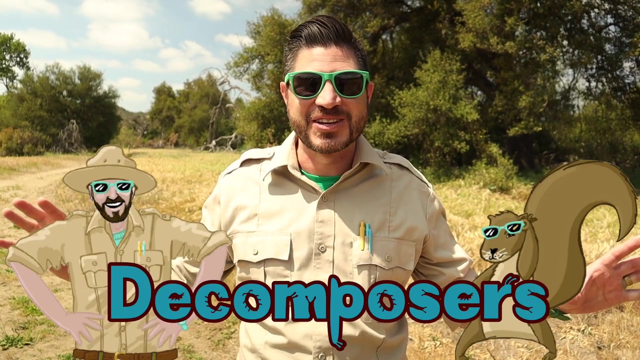 other insects. They have powerful jaws that they'll use to defend their home. Even though ants are a little bit of a nuisance, they're still a very important part of nature. They're what we call decomposers, Which means they help keep the ecosystem clean by eating dead waste. 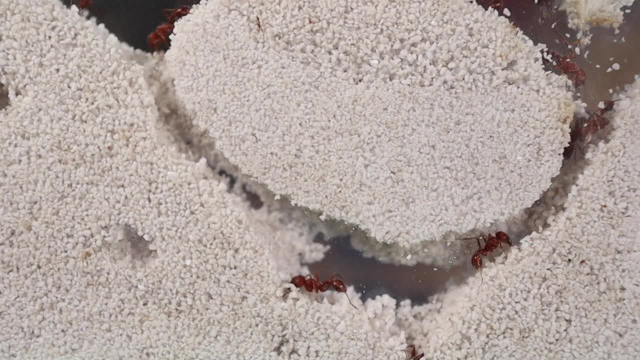 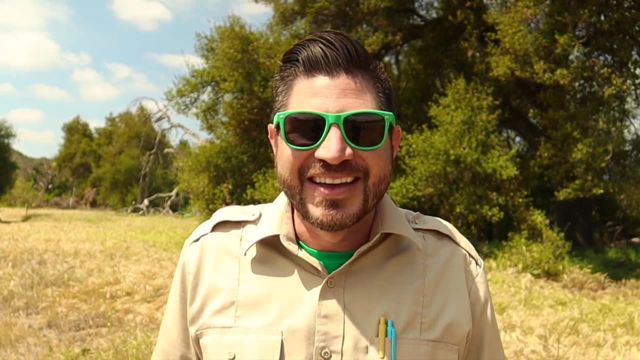 They also introduce air into the soil when they dig their tunnels, and they're an excellent source of food for animals like bears, woodpeckers, other insects and anteaters Cha. They can also help plants grow by taking their seeds deep underground into their colony. 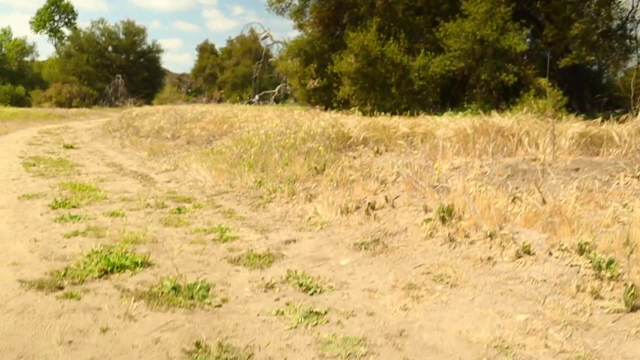 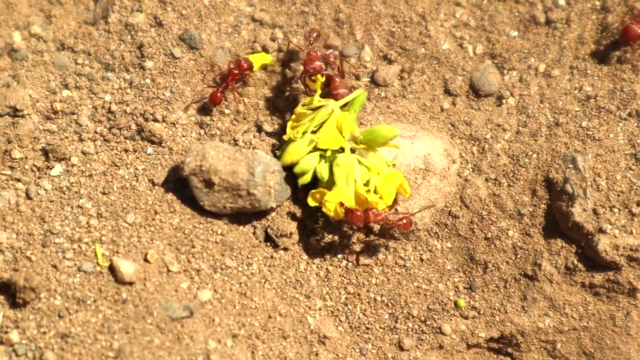 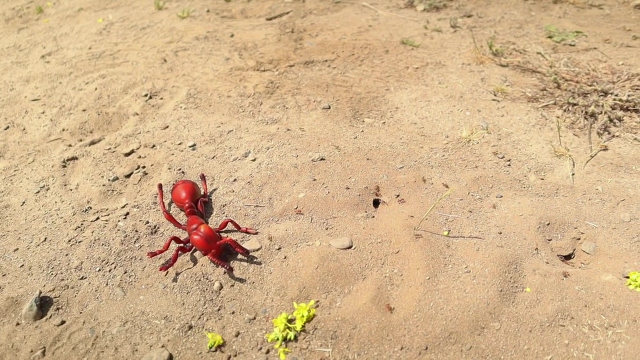 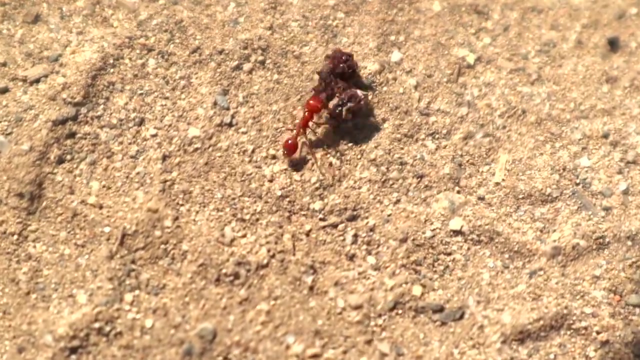 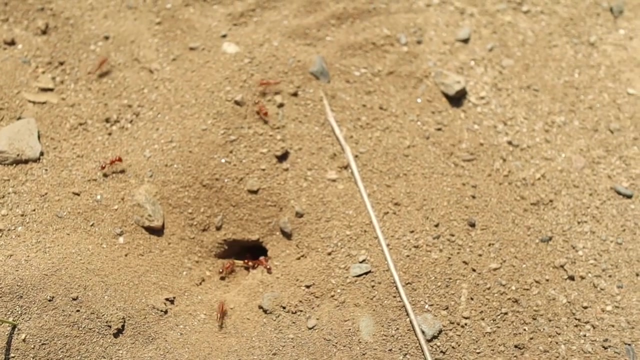 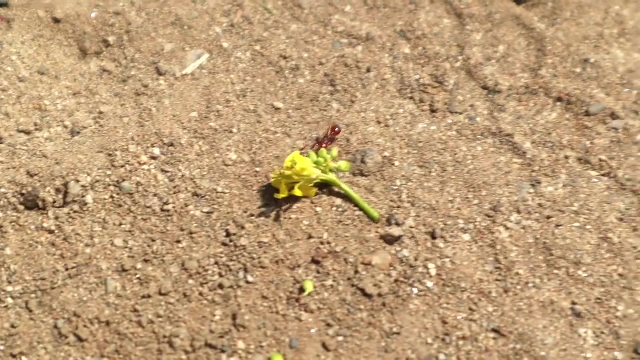 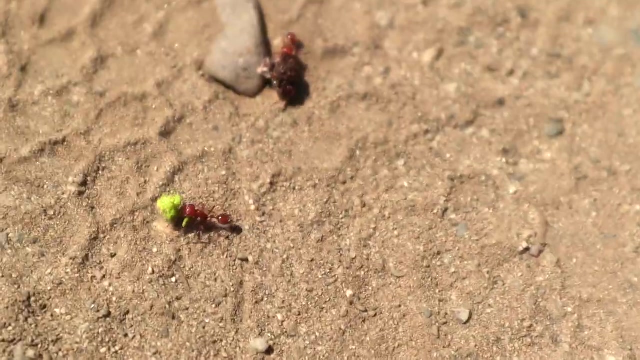 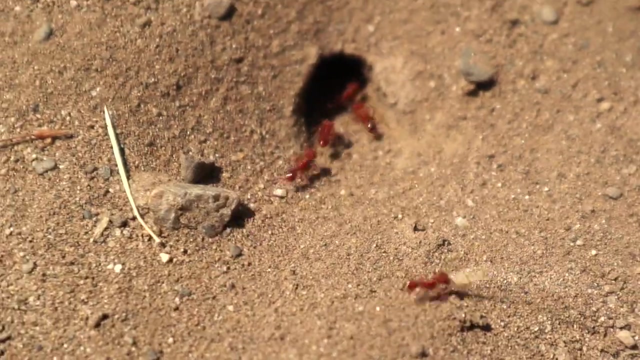 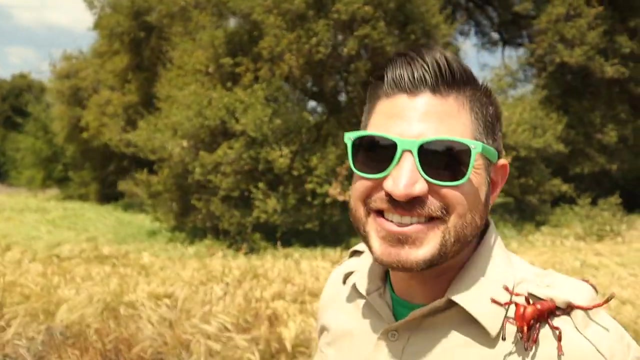 like these harvester ants are doing here. So where do these plants grow? Thank you, Thank you. So the next time an ant crashes your picnic, just invite them to the party, because they're just doing what ants do best. Now let's go back to the ranger station and learn some more. 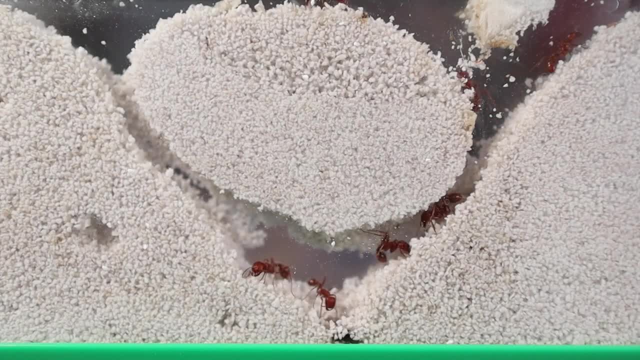 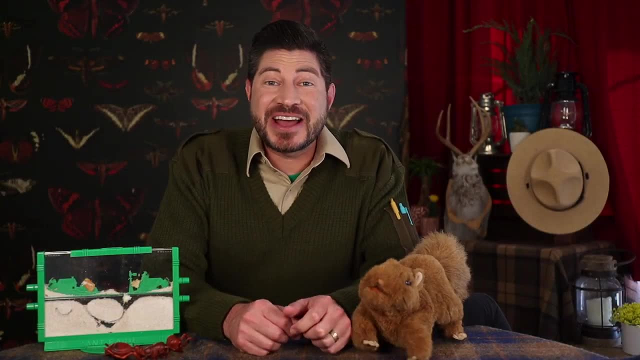 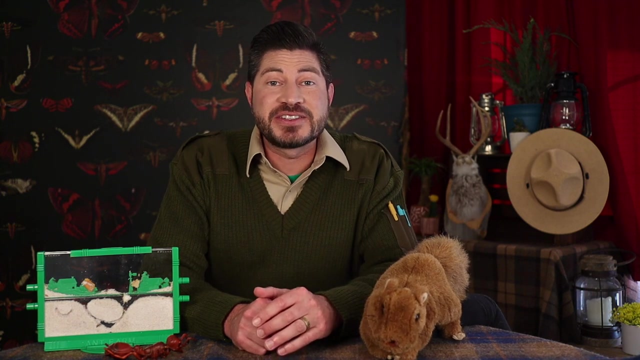 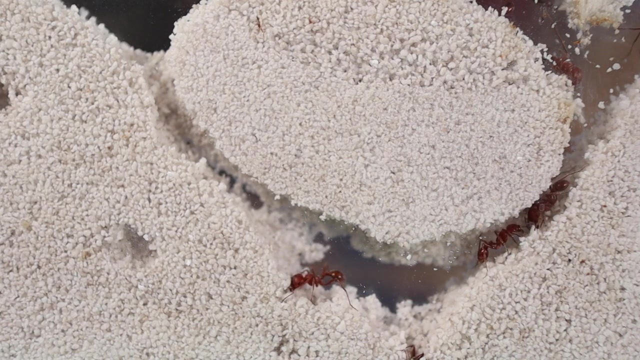 Howdy, junior rangers, Welcome back to the ranger station. I bet you'll never look at ants the same way again. And if you thought making your observations in the wild was fun, consider getting yourself an ant farm like this one. That way, you can make your observations from the comfort of your own home. 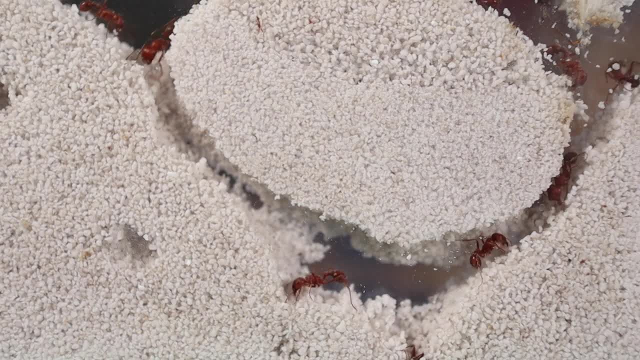 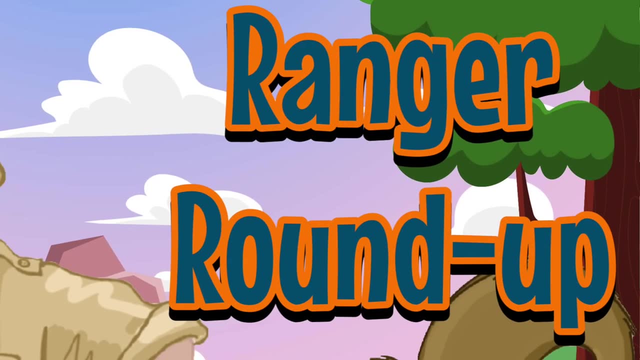 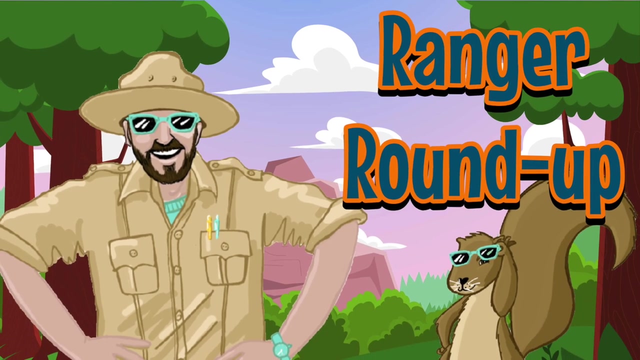 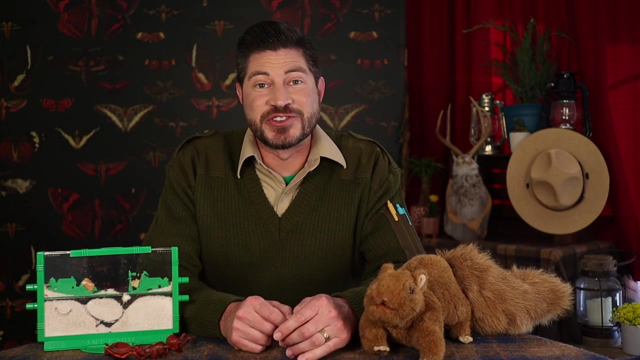 I could watch these sisters build their tunnels forever. Keep up the good work, ladies. You do your thing and we'll do the ranger roundup This week is extra special because we had three junior rangers ask the same exact question: Junior ranger Ivy, junior ranger Lorena and junior ranger Frankie. 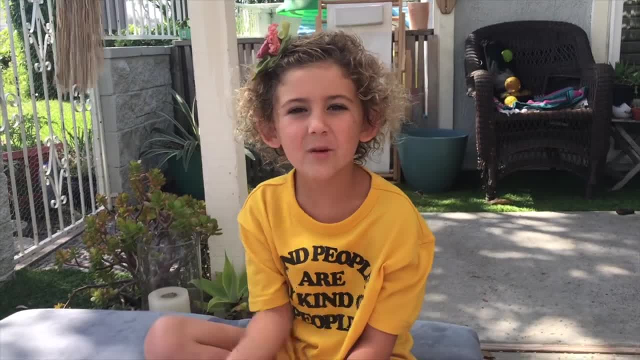 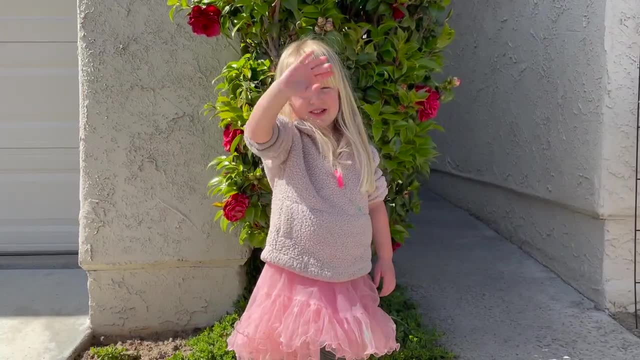 Hi Ranger Zach. I want to know why this guy's blue? Help me see, Hi Ranger Zach. I was just wondering: why is the sky blue? Hi Ranger Zach, What do you want to ask? Why the sky is blue?